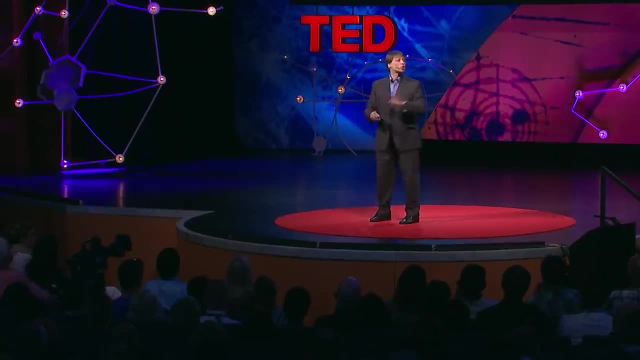 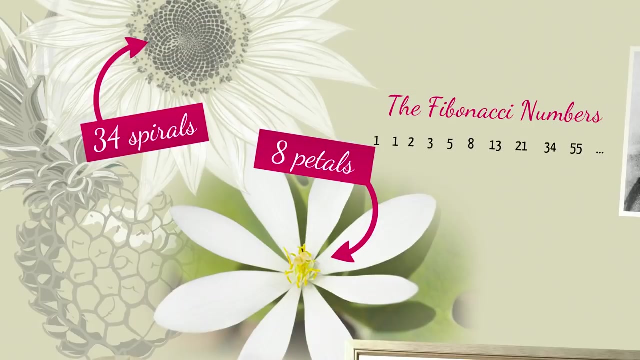 of applications. Fibonacci numbers appear in nature surprisingly often. The number of petals on a flower is typically a Fibonacci number, or the number of spirals on a sunflower or a flower. The number of petals on a flower is typically a Fibonacci number or the number. 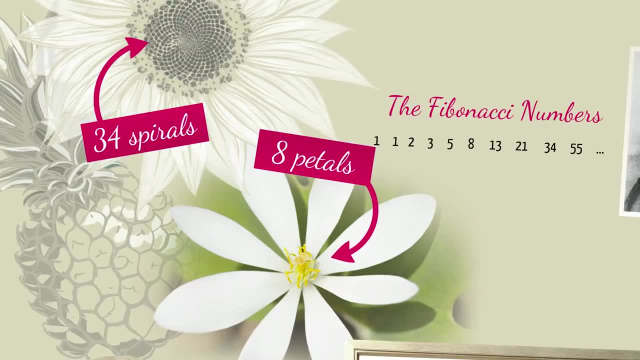 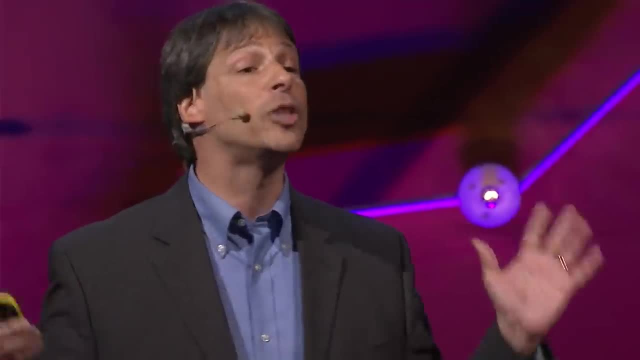 of petals on a pineapple tends to be a Fibonacci number as well. In fact, there are many more applications of Fibonacci numbers, but what I find most inspirational about them are the beautiful number patterns they display. Let me show you one of my favorites. Suppose you, 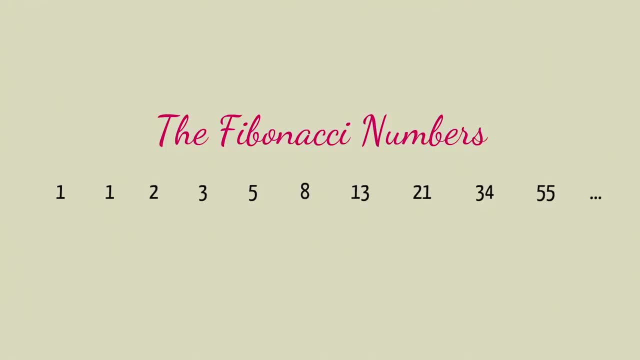 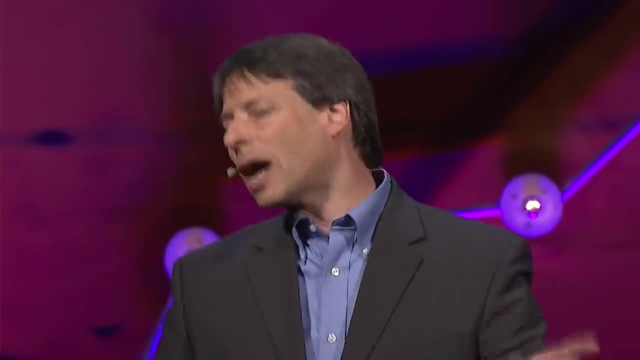 like to square numbers and, frankly, who doesn't? Let's look at the squares of the first few Fibonacci numbers. okay, So one squared is one, two squared is four. three squared is nine, five squared is twenty-five. All right, now it's no surprise that when you add consecutive Fibonacci numbers, you 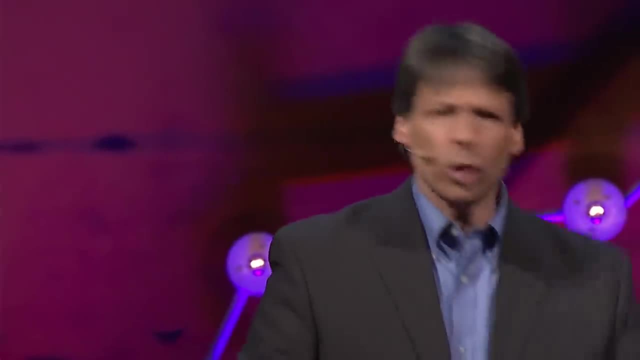 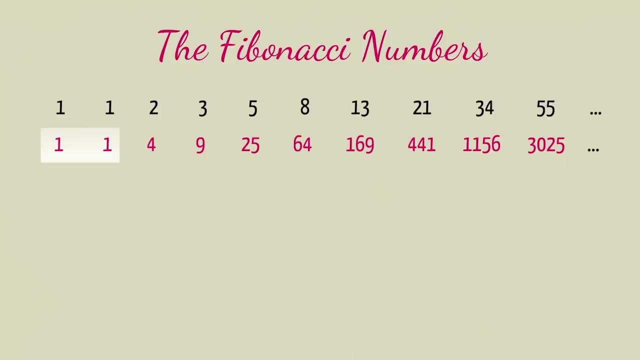 get the next Fibonacci number right. That's how they're created, But you wouldn't expect anything special to happen when you add the squares together. But check this out: One plus one gives us two, and one plus four gives us five, And four plus nine is thirteen nine. 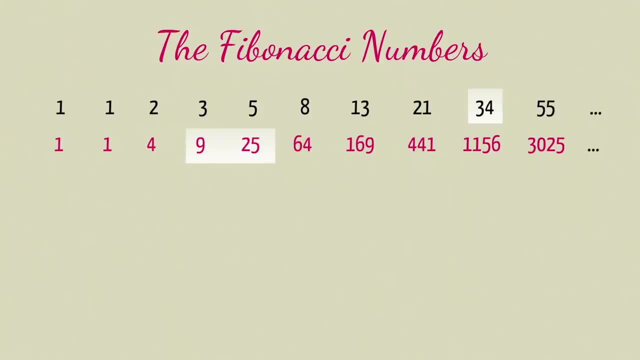 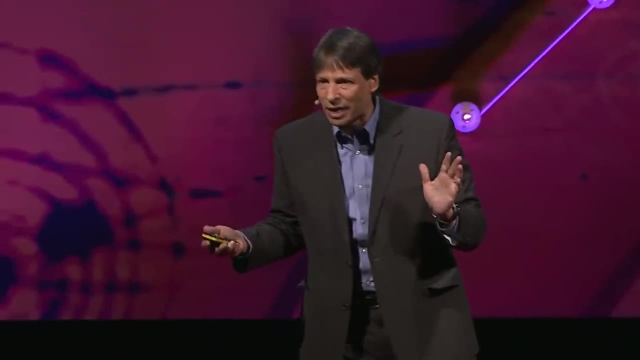 plus twenty-five is thirty-four. and yes, the pattern continues, In fact. here's another one. Suppose you wanted to look at adding up the squares of the first few Fibonacci numbers. Let's see what we get there. So one plus one plus four is six. Add nine to that, we get. 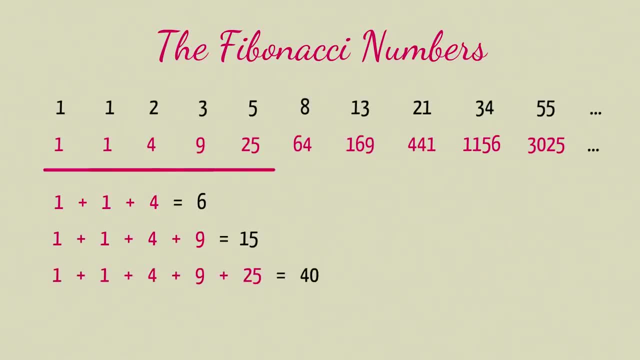 fifteen Add twenty-five, we get forty Add sixty-four, we get one hundred four. Now look at those numbers. Those are not Fibonacci numbers, but if you look at them closely, you'll see the Fibonacci numbers buried inside of them. Do you see it? I'll show it to you. 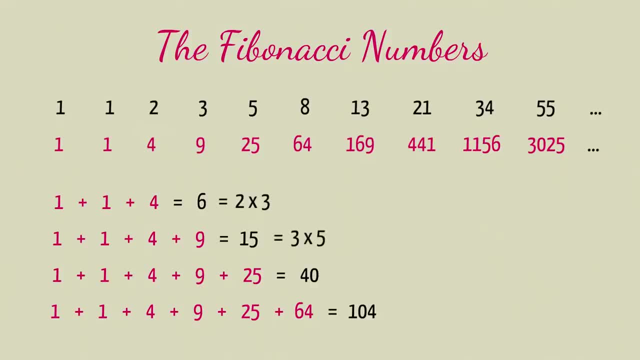 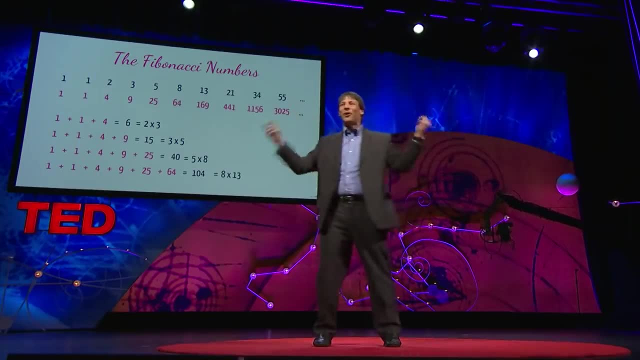 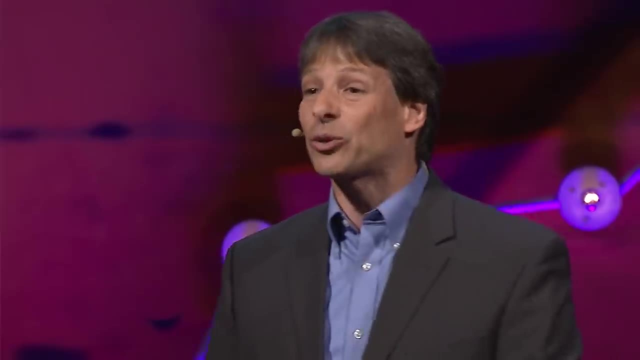 Six is two times three. Fifteen is three times five. Forty is five times eight. Two three five eight. Who do we appreciate? Fibonacci, of course. Now, as much fun as it is to discover these patterns, it's even more satisfying to understand why they are. 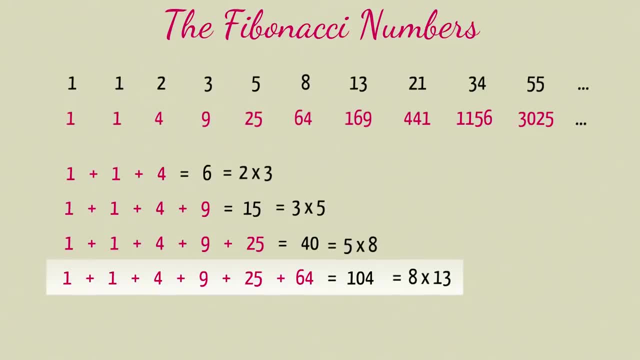 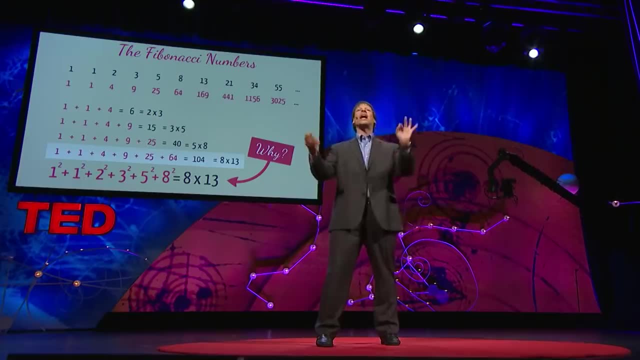 true. Let's look at that last equation. Why should the squares of one, one, two, three, five and eight add up to eight times thirteen? I'll show you by drawing a sequence of squares. Here's a simple picture. We'll start with a one-by-one square and next to that put. 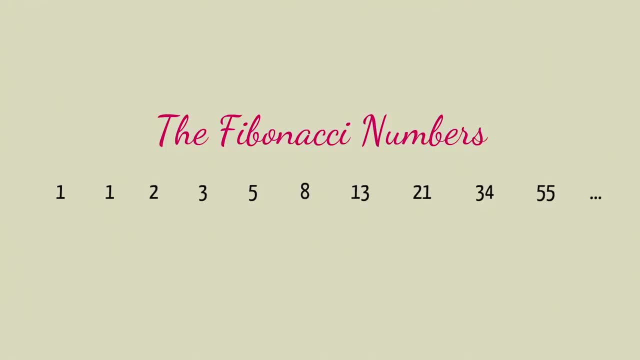 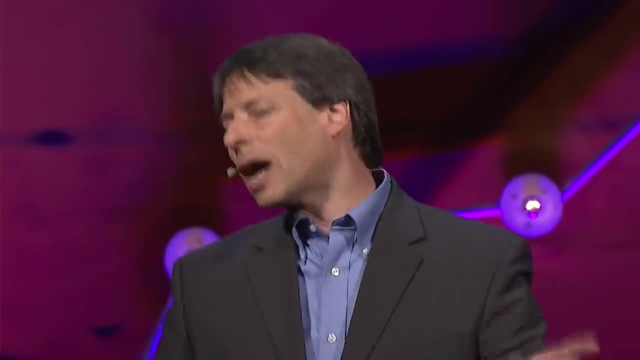 like to square numbers and, frankly, who doesn't? Let's look at the squares of the first few Fibonacci numbers. okay, So one squared is one, two squared is four. three squared is nine, five squared is twenty-five. All right, now it's no surprise that when you add consecutive Fibonacci numbers, you 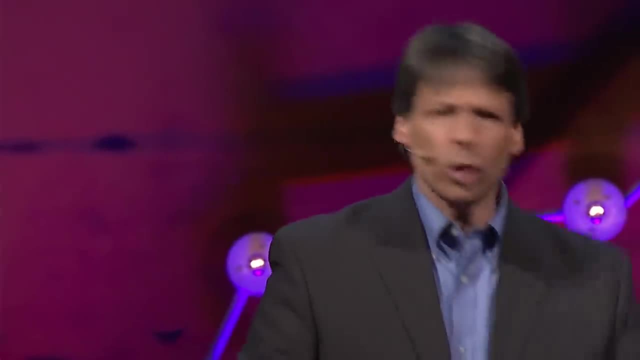 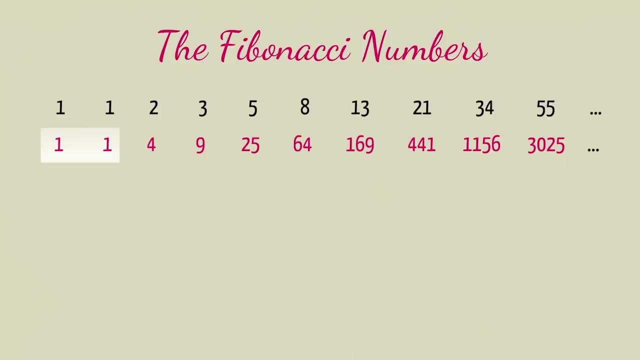 get the next Fibonacci number right. That's how they're created, But you wouldn't expect anything special to happen when you add the squares together. But check this out: One plus one gives us two, and one plus four gives us five, And four plus nine is thirteen nine. 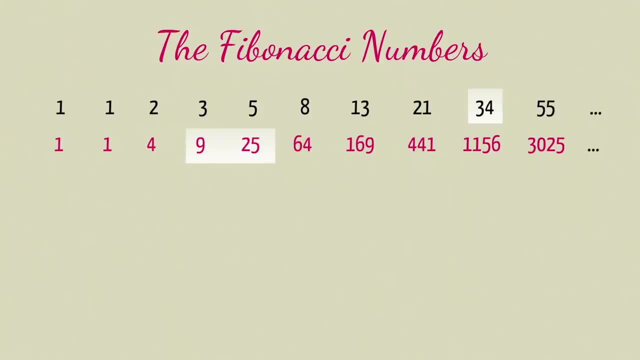 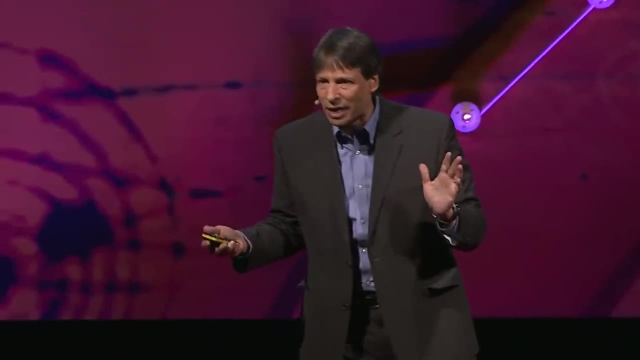 plus twenty-five is thirty-four. and yes, the pattern continues, In fact. here's another one. Suppose you wanted to look at adding up the squares of the first few Fibonacci numbers. Let's see what we get there. So one plus one plus four is six. Add nine to that, we get. 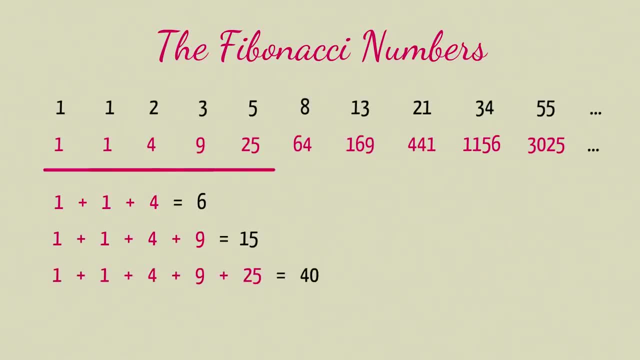 fifteen Add twenty-five, we get forty Add sixty-four, we get one hundred four. Now look at those numbers. Those are not Fibonacci numbers, but if you look at them closely, you'll see the Fibonacci numbers buried inside of them. Do you see it? I'll show it to you. 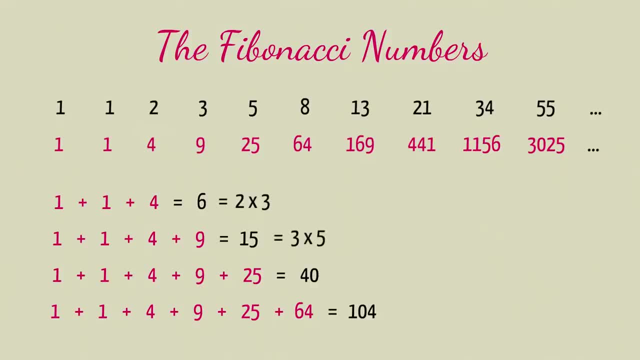 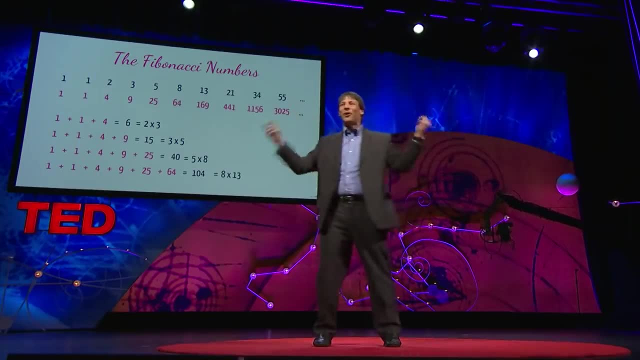 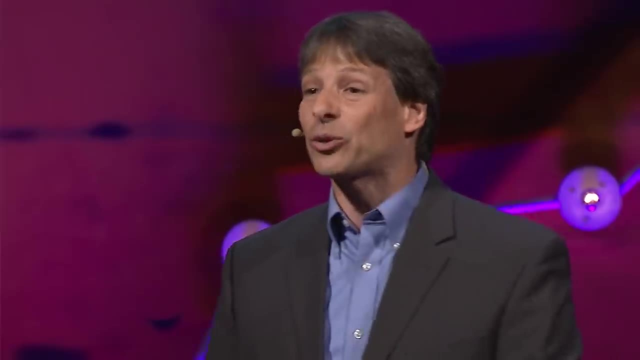 Six is two times three. Fifteen is three times five. Forty is five times eight. Two three five eight. Who do we appreciate? Fibonacci, of course. Now, as much fun as it is to discover these patterns, it's even more satisfying to understand why they are. 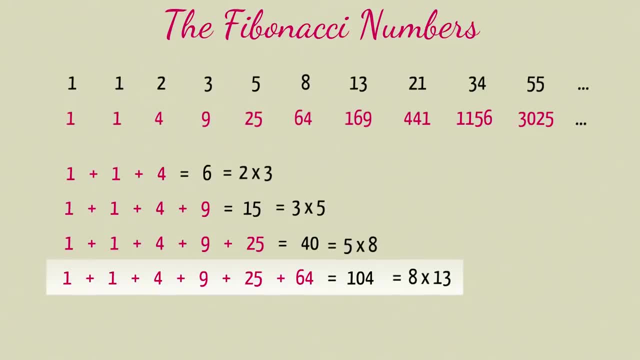 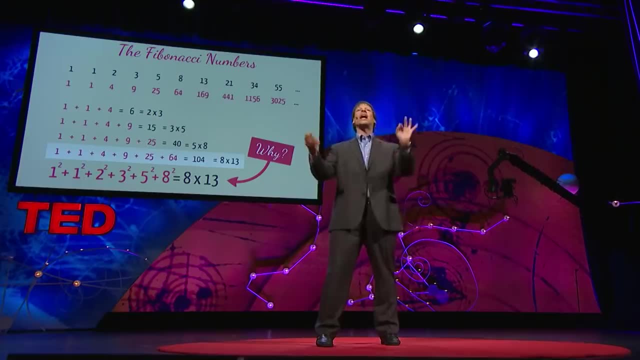 true. Let's look at that last equation. Why should the squares of one, one, two, three, five and eight add up to eight times thirteen? I'll show you by drawing a sequence of squares. Here's a simple picture. We'll start with a one-by-one square and next to that put. 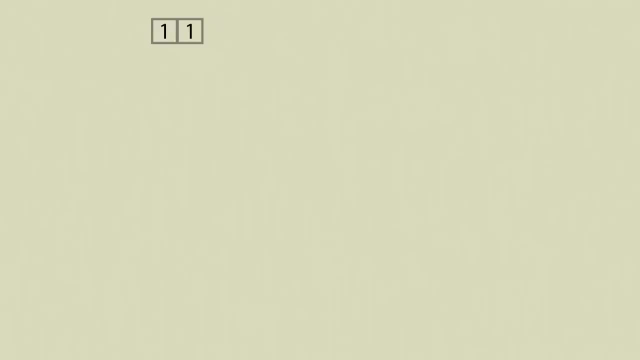 another one-by-one square. Together they form a one-by-two rectangle. Beneath that I'll put a two-by-two square and next to that a three-by-three square, Beneath that a five-by-five square and then an eight-by-eight square, creating one giant rectangle right. 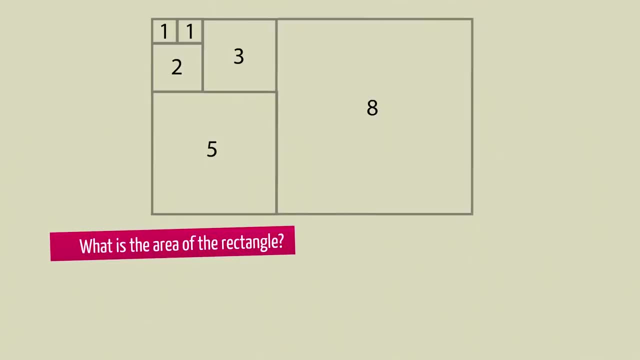 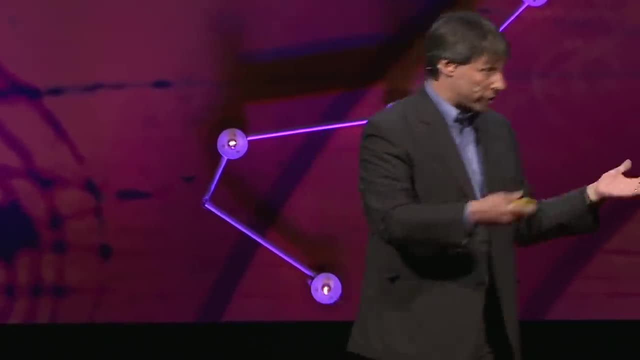 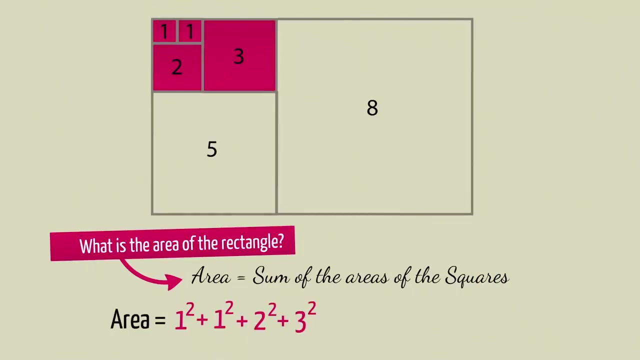 Now, let me ask you a simple question: What is the area of the rectangle? Well, on the one hand, it's the sum of the areas of the squares inside it. right, Just as we created it, It's one squared plus one squared plus two squared plus three squared plus five. 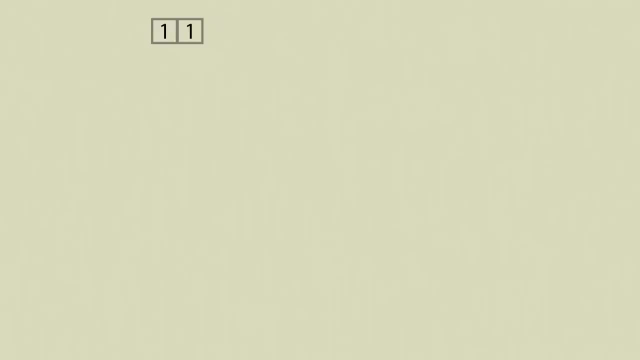 another one-by-one square. Together they form a one-by-two rectangle. Beneath that I'll put a two-by-two square and next to that a three-by-three square, Beneath that a five-by-five square and then an eight-by-eight square, creating one giant rectangle right. 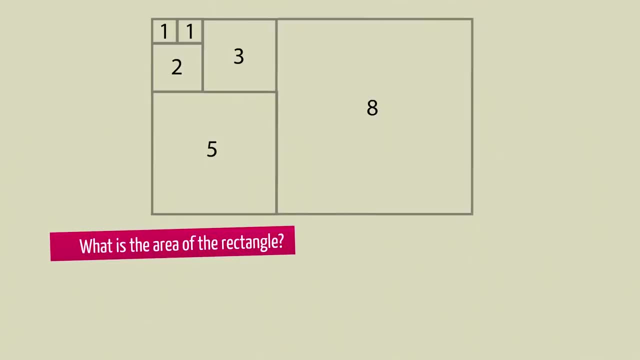 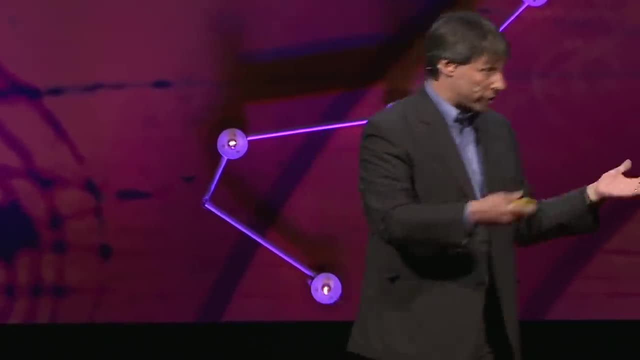 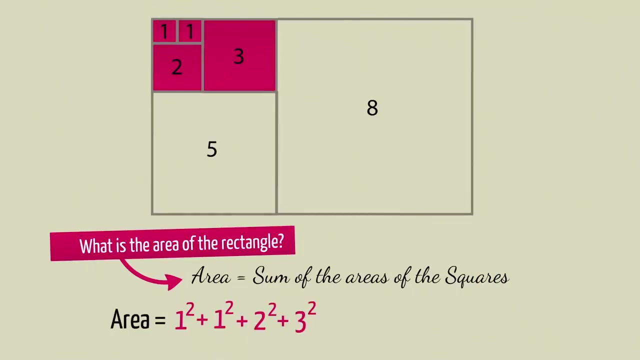 Now, let me ask you a simple question: What is the area of the rectangle? Well, on the one hand, it's the sum of the areas of the squares inside it. right, Just as we created it, It's one squared plus one squared plus two squared plus three squared plus five. 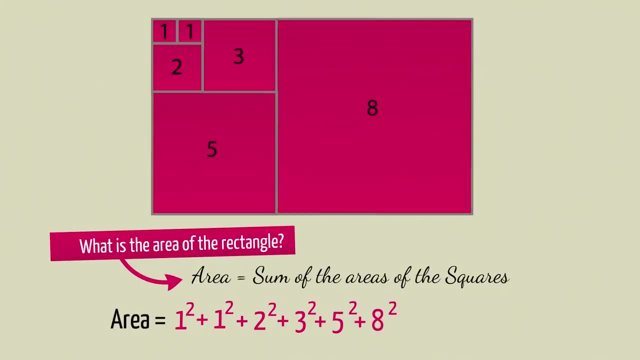 squared plus eight. squared right, That's the area. On the other hand, because it's a rectangle, the area is equal to its height times its base, And the height is clearly eight, and the base is five plus eight, which is the next Fibonacci number, thirteen. We 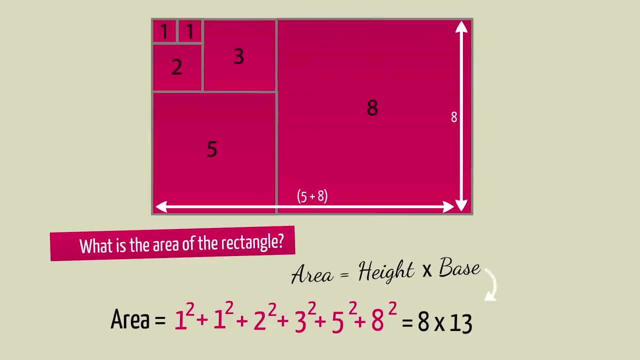 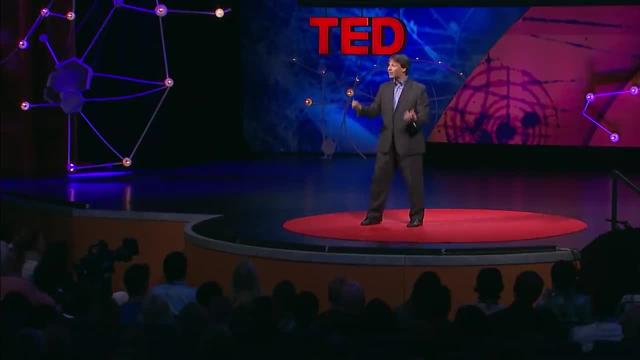 right. So the area is also eight times thirteen. Since we've correctly calculated the area two different ways, they have to be the same number, And that's why the squares of one, one, two, three, five and eight add up to eight times thirteen. Now, if we continue, 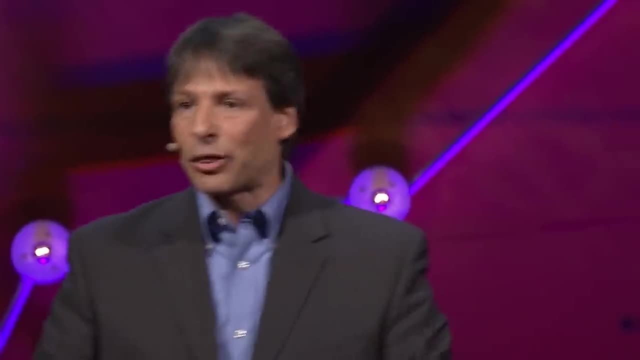 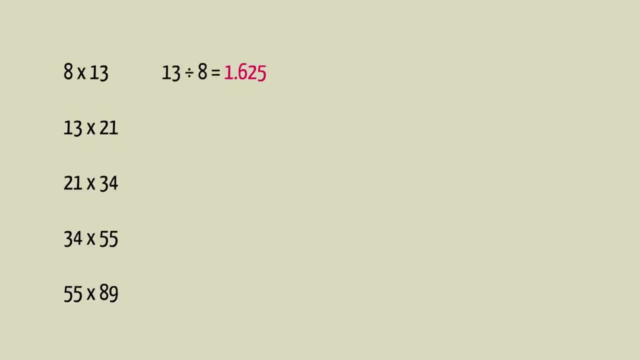 this process, we'll generate rectangles of the form thirteen-by-twenty-one, twenty-one-by-thirty-four, and so on. Now check this out: If you divide thirteen by eight, you get one point six-two-five. And if you divide the larger number by the smaller number, then these ratios get closer. 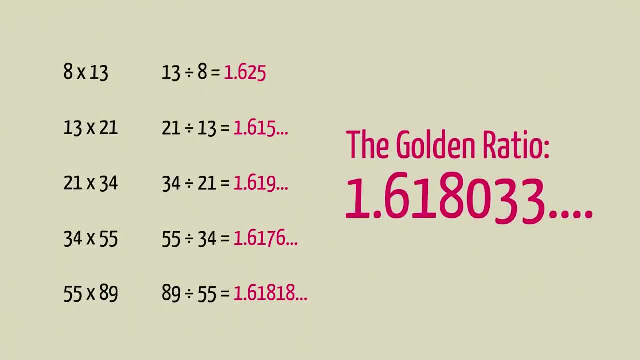 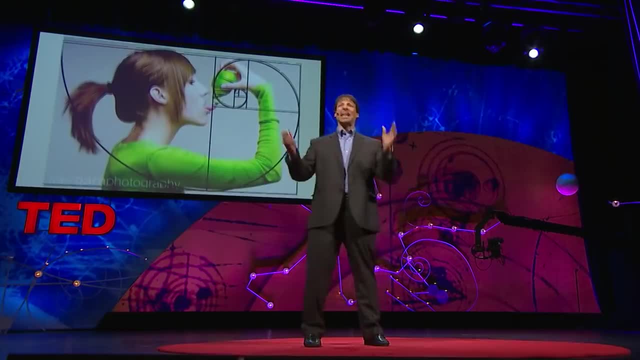 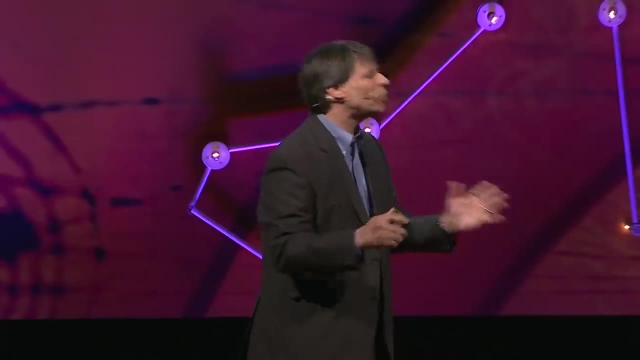 and closer to about one point six-one-eight, known to many people as the golden ratio, a number which has fascinated mathematicians, scientists and artists for centuries. Now I show all this to you because, like so much of mathematics, there's a beautiful side to 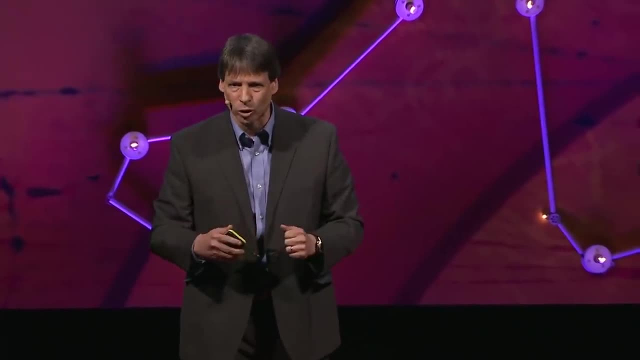 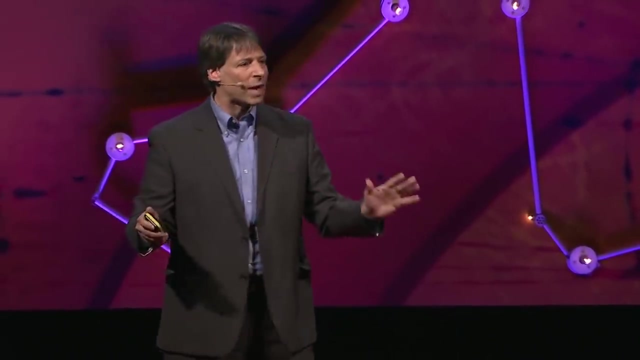 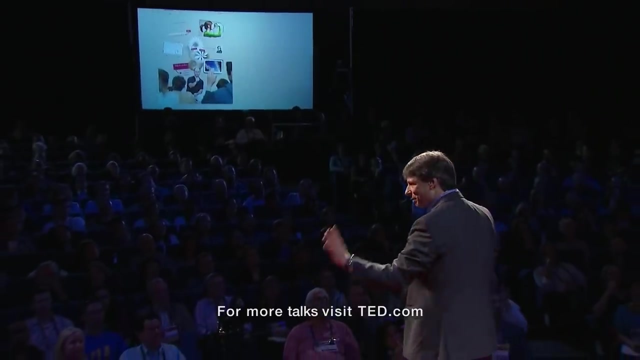 it that, I fear, does not get enough attention in our schools. We spend lots of time learning about calculation, but let's not forget about application, including perhaps the most important application of all: learning how to think. If I could summarize this in one sentence, it would be: 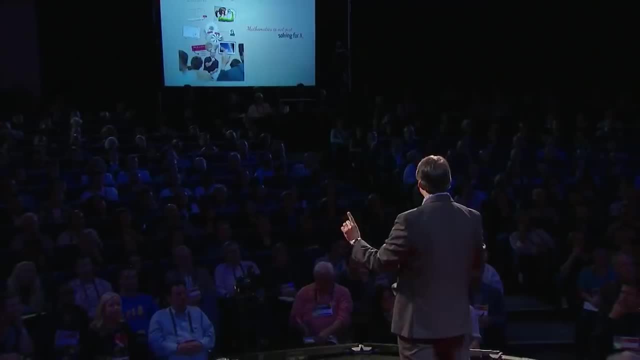 this Mathematics is not just solving for x, it's also figuring out y. Thank you very much.